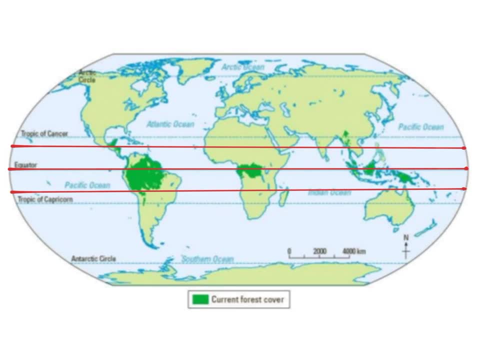 within this band marked on the map. This narrow area either side of the equator is contained within the tropics, being south of the Tropic of Cancer and north of the Tropic of Capricorn. At the equator we receive the most solar insulation because of the curvature of the earth. 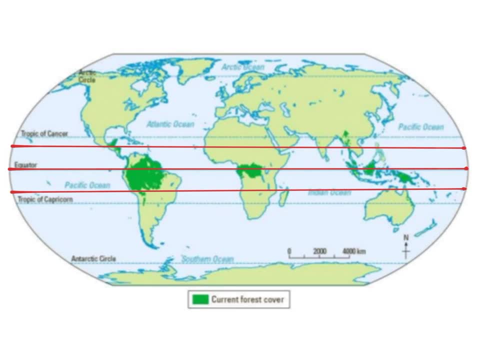 This means that, per square metre, the equator receives the greatest amount of solar radiation. Because it is warm at the equator, it causes the ground to heat up. As the ground heats up, it warms the air above it. As the air warms, it becomes less dense and it starts to rise. 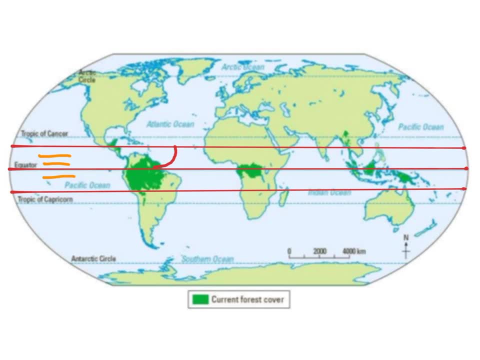 The air will continue to rise until it starts to cool because of the altitude, at which point it will start to fall. This will happen in both the north of the equator and it will happen at the south of the equator. We call this the Hadley Cells. 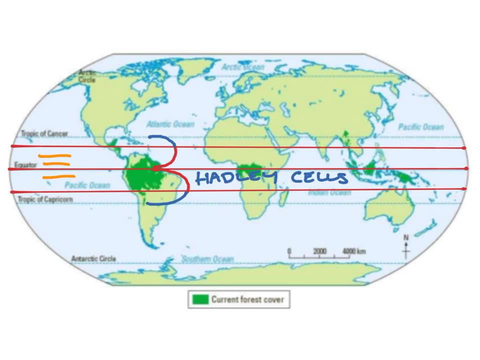 Where we have air rising or our rising limb of the Hadley Cells, we get low pressure, because the air is not pushing on the ground but instead is rising. Where the air of the Hadley Cell is falling or the falling limb, we get high pressure. 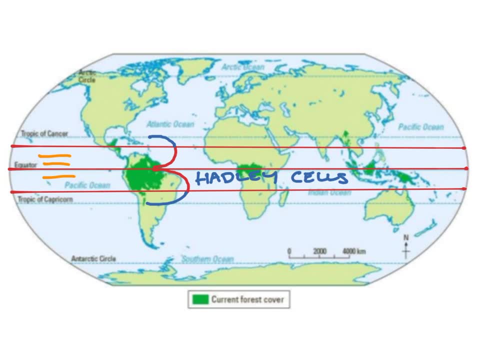 And this is located at the Tropic of Cancer and the Tropic of Capricorn. Low pressure areas see air rising. As the air warms, it rises Where it eventually starts to cool. As it cools, the water vapour contained within the air starts to condense and clouds are formed. 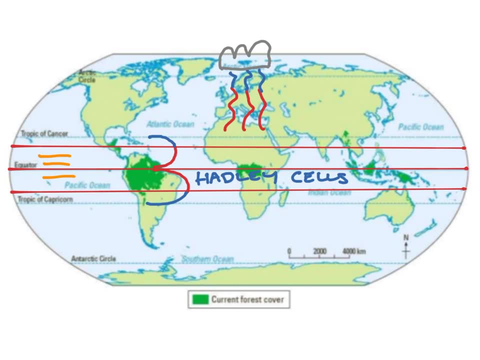 Where we get clouds, rain follows, And throughout the narrow zone where we find tropical rainforests, we get significant amounts of precipitation in the form of rain. The two factors of the heat caused by the equator being located at zero degrees latitude and the